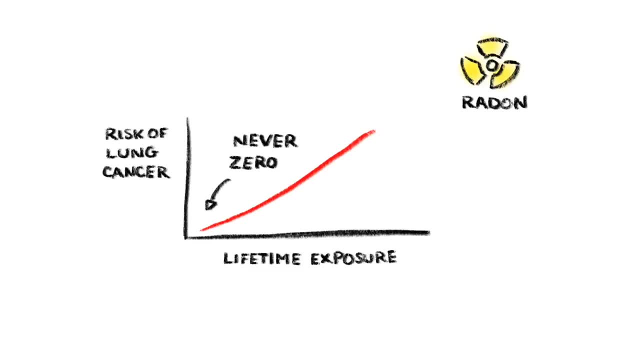 protection specialists recommend levels in homes are kept as low as you can reasonably get them. But what's the answer? What does this mean? if you find yourself living somewhere with high radon levels In the US, the Environmental Protection Agency recommends you take action to reduce radon. 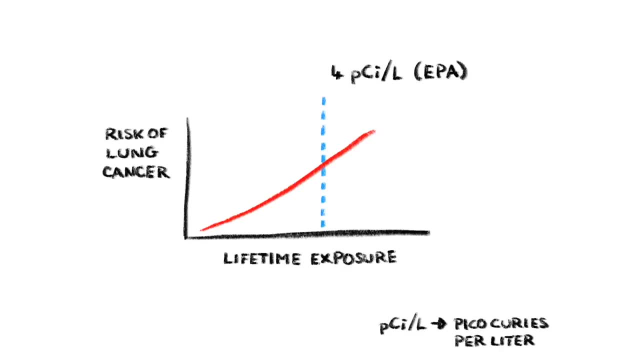 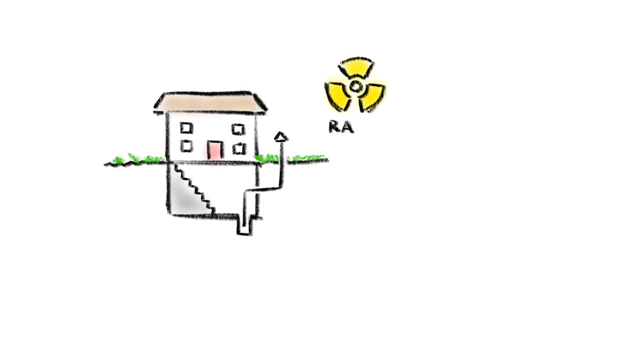 levels if they're above 4 picocuries per litre. The World Health Organisation is a little bit more conservative here and suggests you do something about it if the levels are above 2.7 picocuries per litre. The good news, though, is that for most people it's not too hard to get indoor concentrations. 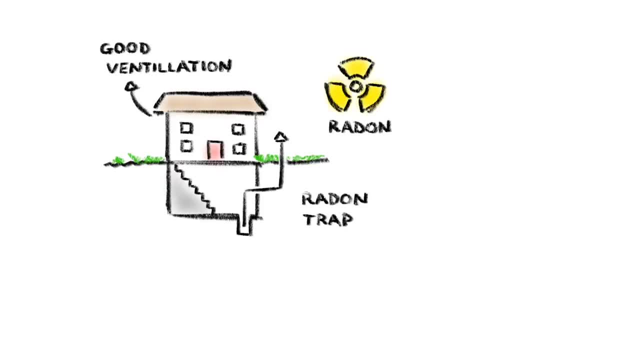 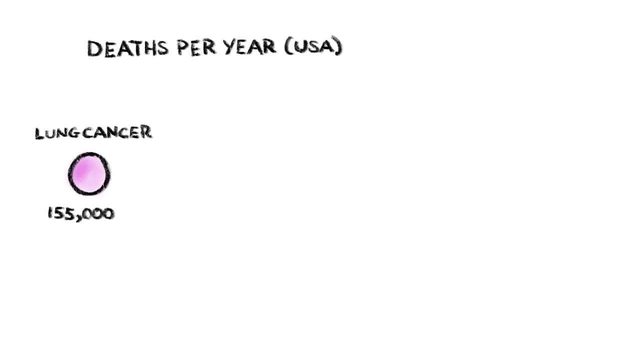 below the EPA action level. But if you are stuck with high radiation levels, how do you know what the additional risk is? To get a handle on this, we need to look at the chances of being killed by this invisible gas Each year. in the US, around 155,000 people a year die from lung cancer. 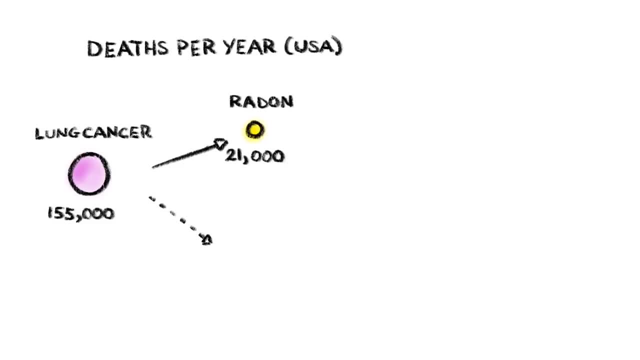 And of these, something like 21,000 deaths are associated with radon. Many of these, though, are also connected with smoking separating out the non-smokers. Around 2,900 people a year die from lung cancer, And around 1,000 people a year die from radon-related lung cancer. 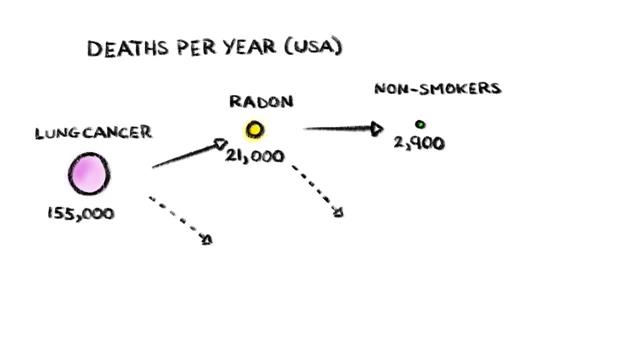 This is a serious number of deaths, But because of the number of people living in the US, the actual risk of dying from radon exposure in any given year is not that high. On average, something like 9,000 people out of every million in the US die each year. 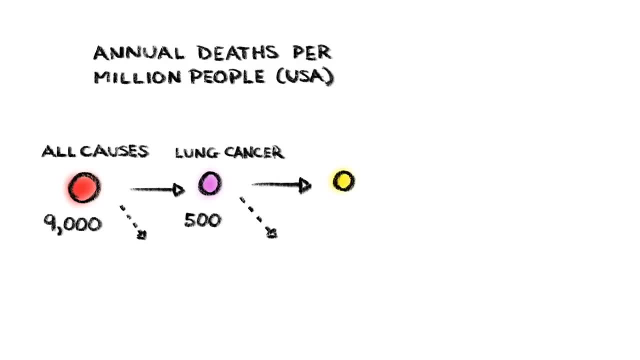 500 people out of every million die from lung cancer And 70 people out of every million die because they've been exposed to radon for a number of years. But when you ever think about it, you can't really think about that. 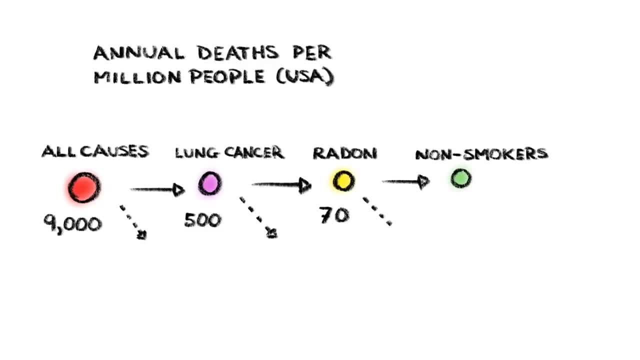 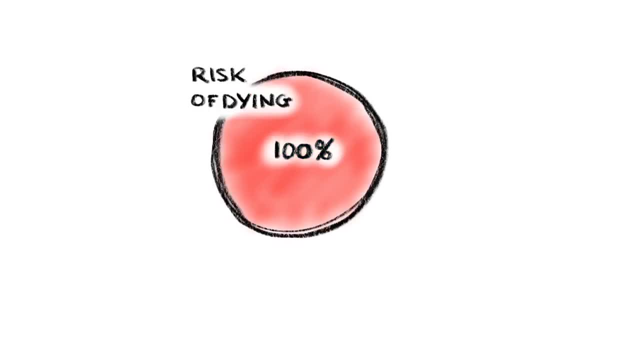 If you only consider people who don't smoke, only 10 people out of every million die from radon exposure. Another way of looking at this is to ask what the chances are that, when you die, radon was the cause. And here it turns out that when you pop your clogs, there's around about a 1 to 2 in 1,000. 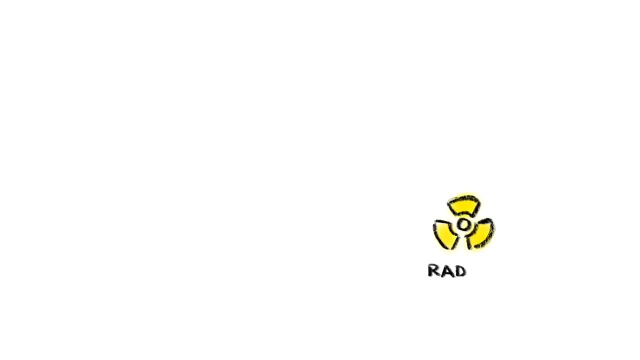 chance that radon will be to blame. It's somewhat comforting to know that if you're inhaling radon, the chances are that something else will kill you first, But this doesn't answer the question of how much safer you'll be if you reduce your radon.